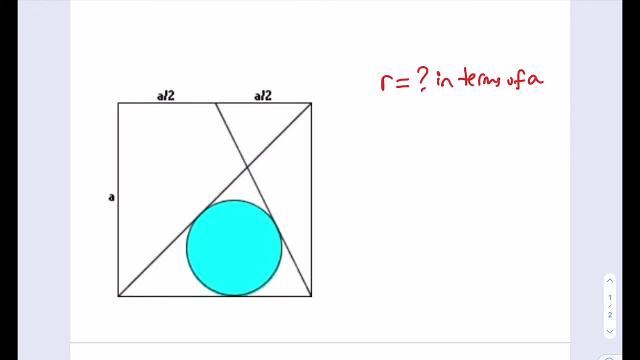 triangle. So we're going to find the side lengths of this triangle, How We're going to take advantage of symmetry. Right, We're actually going to be using similarity here, So let's go ahead and do that. So how does that work? So suppose this is A, this is B, this is C, this is D, this is E. 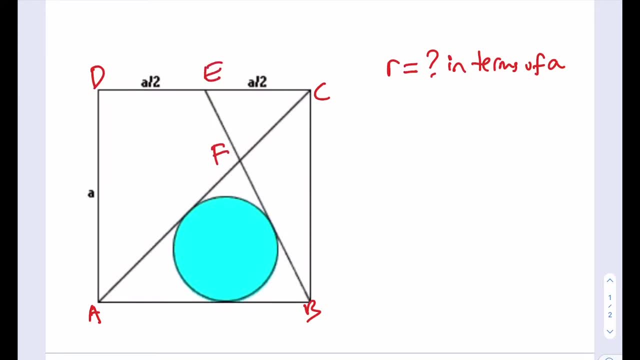 and this is F. So I'm just saying that triangles A, B, F and C, F, E are similar, And the similarity ratio is actually going to be two to one. So what that means is that we can find the side lengths if needed, or we can actually find something more interesting, which is the 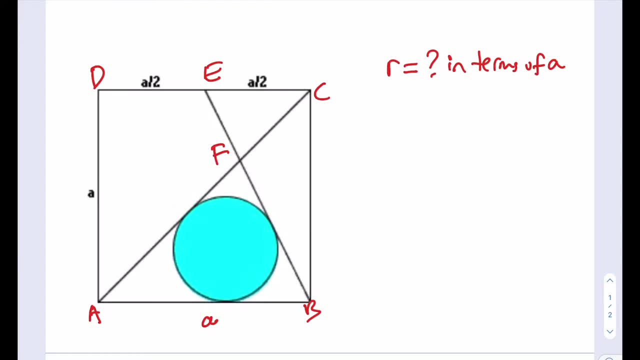 height. Now, why do we need the height? So let's go ahead and outline the solution here. We're going to go ahead and find the height of triangle A- F, B and then, using the height and the base, we're going to find the area of triangle A- F, B. And how does that work? So we're going to find the 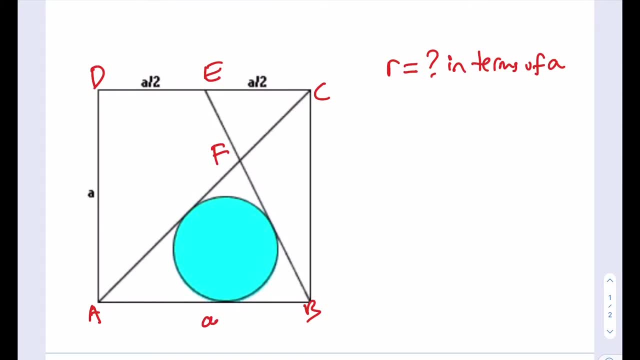 height in this hair It has thewhole. Where do you find the height angle I have here in? here is the side length. So here we're going to group down the sides and then, at the base of that, the side length is further away from the height. So it's the norm, Right? The entre builder actually. 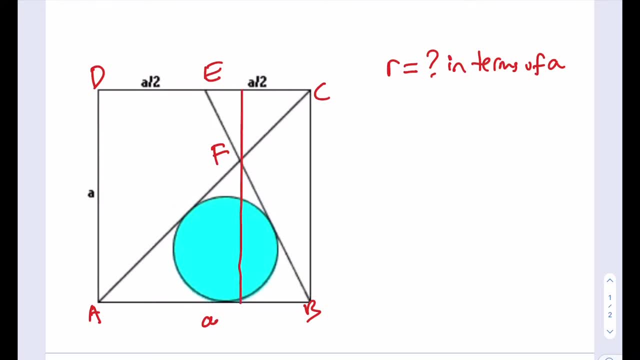 has the center line, because this is the 까. The first thing is to put this here. It's an integral. the integral of the highest to lowest is the integral of the nest. So I'm going to type this in the chapter column in here. ok, so it's 2 and 3px around. This is the increasing expression of height value. but there is noاه, there is noaah, there is noah and, like I was telling you, the saleit, this is the. 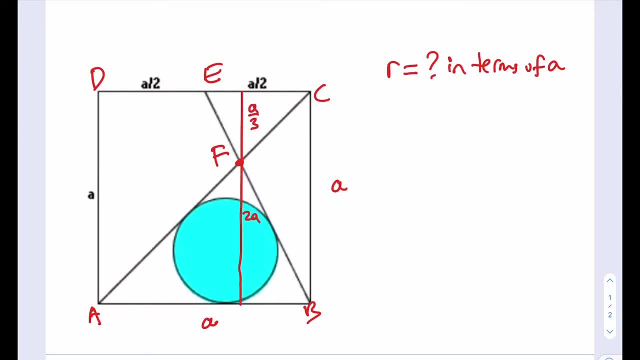 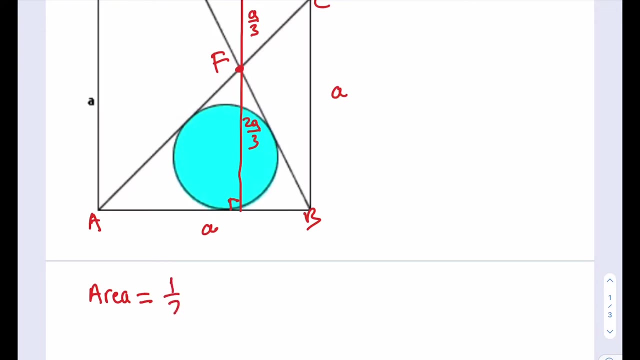 this is going to be a over 3 and this is going to be 2a over 3 with the height of the lower triangle. now i'm going to go ahead and write the area from here. okay, so the area of the triangle abf is equal to one half times base times height. okay, the two cancels out and we get from here. 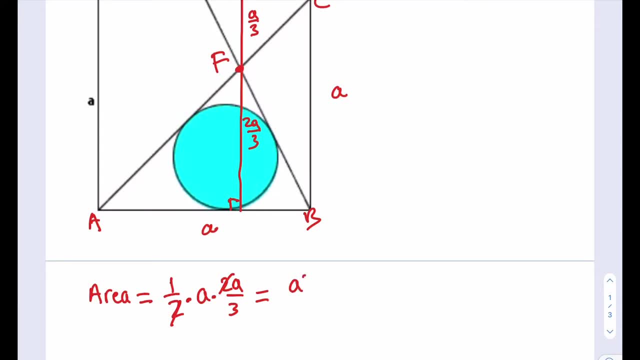 a squared over 3. so the area of triangle afb is a squared over 3. now, how does that help us? well, if the radius of the circle, which is the in radius, is r, then we have this interesting relationship. we can find the area using the in radius. how well, if you multiply the perimeter. 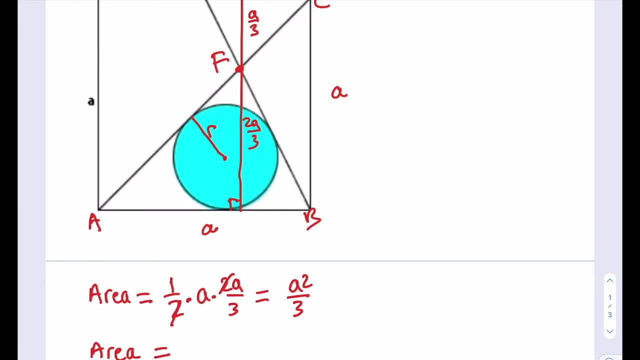 by the radius, you're going to find twice the area. In other words, the area is equal to semi-parameter multiplied by the in radius. That's what we need. So what is the semi-parameter? Well, the semi-parameter is going to be the side lengths added up and then divided by 2.. So let's go ahead and do that. What are the? 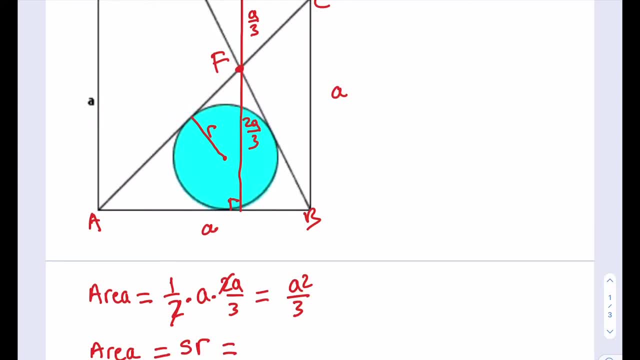 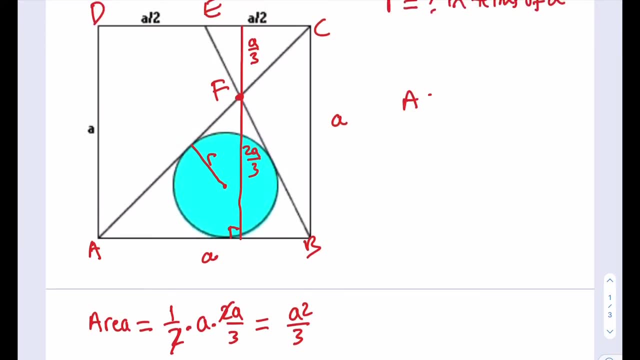 side lengths. Okay, then we need to find AF and FB. How do you find AF and FB? Well, AC is the diagonal, which is a root 2 right, and AF is going to be two-thirds of that, So it's just going to be 2. 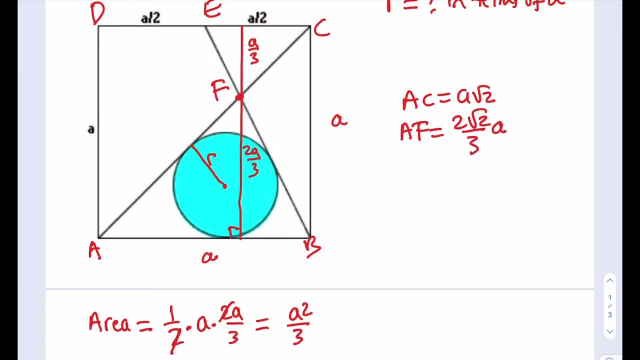 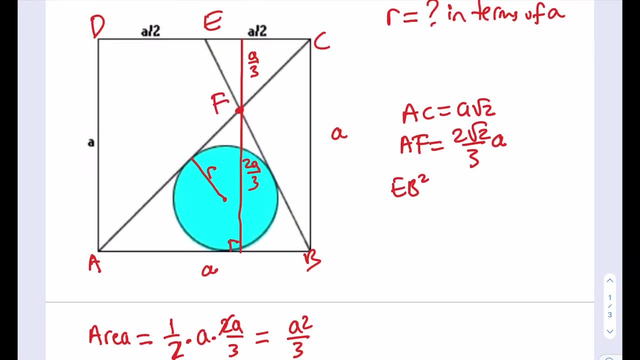 root 2 over 3 multiplied by a. Okay, so we can find EB from Pythagorean theorem. As you know, EB is the hypotenuse of ECB, So EB squared is equal to a squared over 4 plus a squared. From here we get. 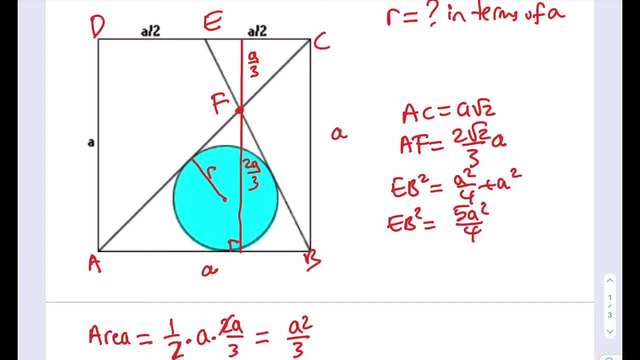 EB squared is equal to 5 a squared over 4 and EB is the diagonal. So we need to find EB, So we need going to be root 5 over 2 times a. now we do know that fb is going to be two-thirds of this. let's 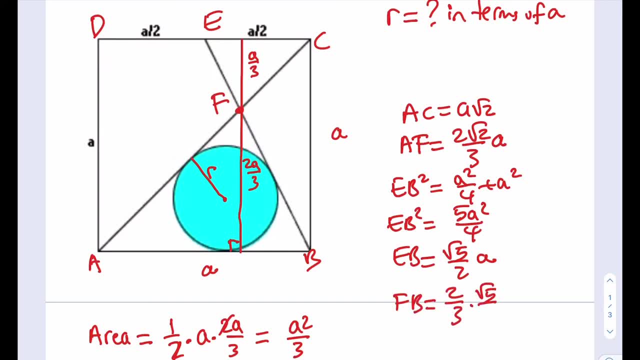 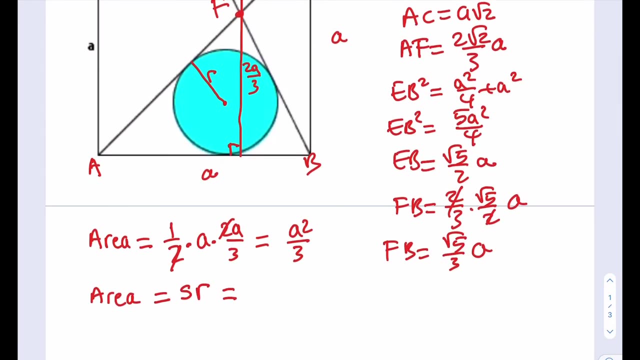 go ahead and multiply this by two-thirds and that's also going to simplify. so fb is going to be root 5 over 3. multiply by a. now we got fb, we got af, we got ab, we can find the semi-perimeter. the semi-perimeter is just going to be the sum of those lengths right, which we found. 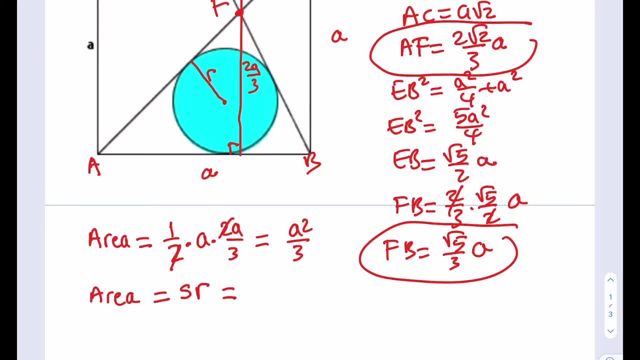 and then fb, and then ab, which is a right. ab is equal to a here. awesome. let's go ahead and plug those in. for for the semi-perimeter we're going to be getting, let's go ahead and write it down here. i'm going to have 2 root 2 over 3 a, plus root 5 over 3 a.